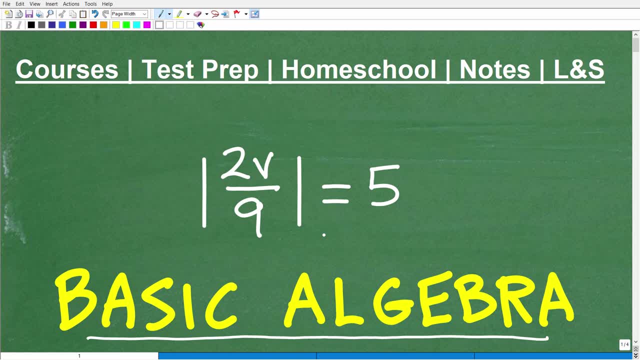 to this problem in just one second. But before we get going, let me quickly introduce myself. My name is John. I'm the founder of TC Math Academy. I'm also a middle and high school math teacher. I have been teaching math for decades. I absolutely love helping people learn mathematics, And I'm going to tell you right now: all of you can be successful in math, And I'm especially speaking to those of you that have a tough time with mathematics. Okay, so, if math is your nemesis, if you're like I hate math, I'm, I'm just 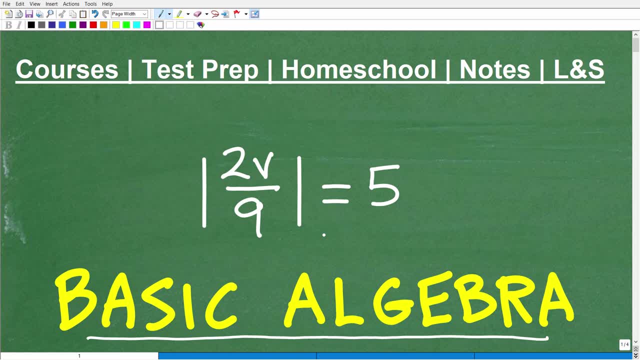 bad at math. Listen, let's see if we can't turn this around. Okay, I'm telling you right now, you definitely can. You can do far better than just pass your course. you can actually excel in math. And if you don't like math, you could even turn that around and end up eventually loving math. But here's the three things you need to be successful in mathematics. One: you got to realize that you got to put in the work. Okay, you need a strong work ethic. There are no shortcuts. there are no easy paths. So if you're not working that hard to learn the material, 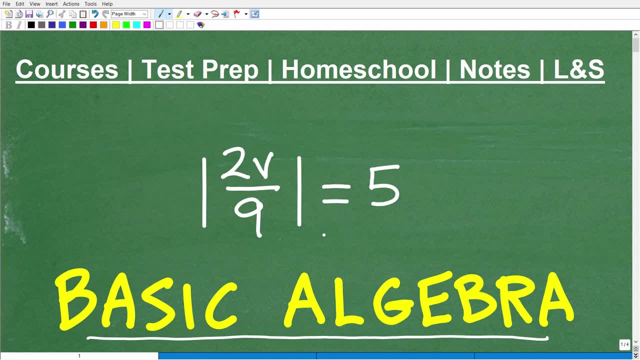 you know you need to work harder. So that's the first thing. The second thing you need is encouragement. All right, you need someone to tell you, telling you, don't give up, especially when math becomes difficult, because there is a path forward. But here's the third thing. you need, probably the most important thing, And that is you need great math instruction. So whoever you're learning from, or whatever you're learning from, you actually have to understand what's being taught. Okay, there's nothing more frustrating than sitting in the classroom- And I'm not trying to knock. 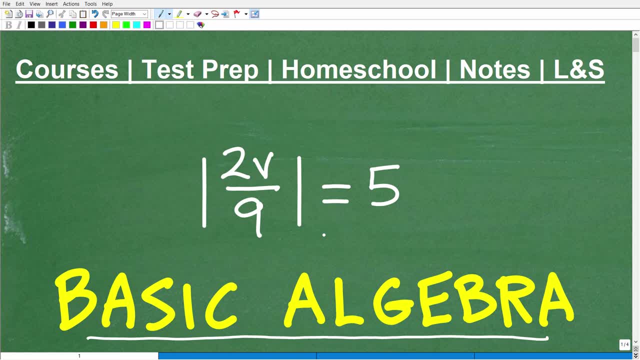 any teachers out there. But if you're not understanding your teacher or if you're not understanding what program you might be using, well, then you're never going to learn right The way I like to teach math, because math is such a technical subject. I like to just explain things. 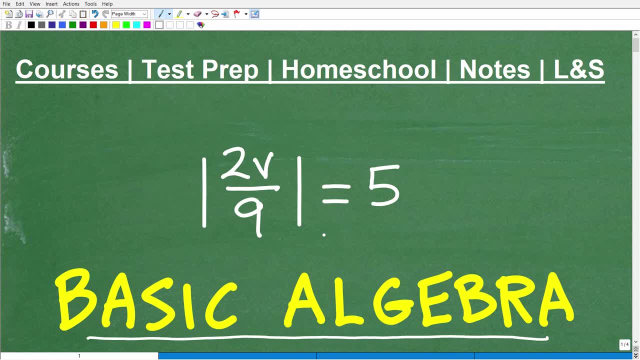 in easy to understand language so everyone gets what's going on without watering down the material. Okay, and I can do that because I've been teaching for years and years And you just get that kind of experience and those kind of skills if you will. But if you need, 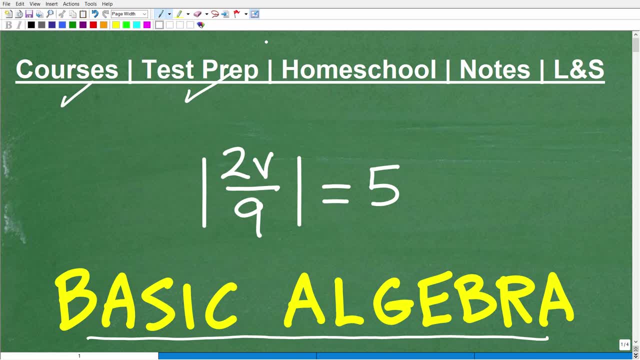 help in your current math course or maybe some sort of special test that you're studying for that has math on it. I'm talking about things like the GED, SAT, ACT, maybe a teacher certification exam, or, if you're homeschooling mathematics, check out my math help program. I'm going to 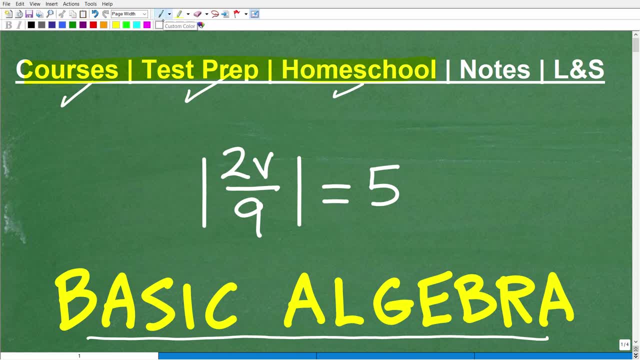 leave a link to it in the description of this video. I literally have over 100 plus different math courses that span these categories and much, much more. I'm also going to leave links to my math notes in the description as well. Most students take average notes- a lot of students. 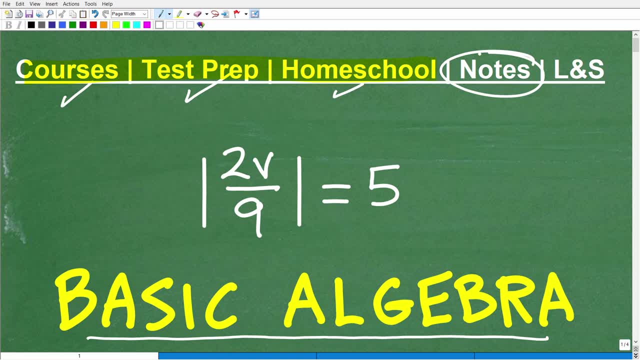 don't take any notes. okay. That is absolutely a recipe for disaster. Students who take great math notes almost always end up with great math grades, So the first thing you need to do is start improving your notes. if your notes are so-so, but you can use my notes in the meantime if you like And if this video helps you. 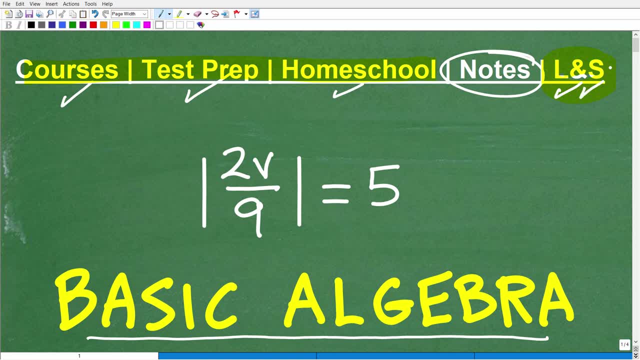 out. don't forget to like and subscribe, as that definitely helps me out. Okay, so what are we talking about here? Well, I'm saying basic algebra. This is a typical type of problem that you could very well see like in a pre-algebra course. 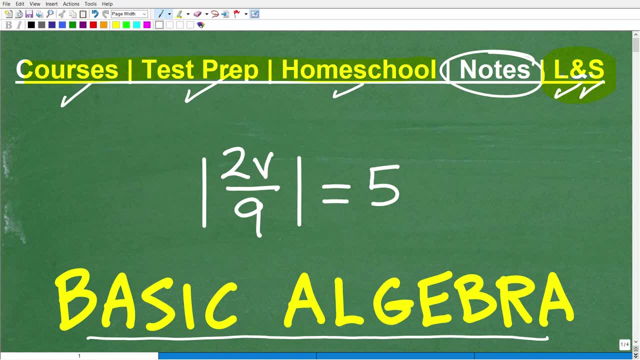 Certainly like an Algebra 1 course, and what we're dealing with here is absolute value. So these little bars right here are indicating this is an absolute value function. Okay, and what is absolute value? I want to explain all this in a second, but this happens to be an absolute value equation. 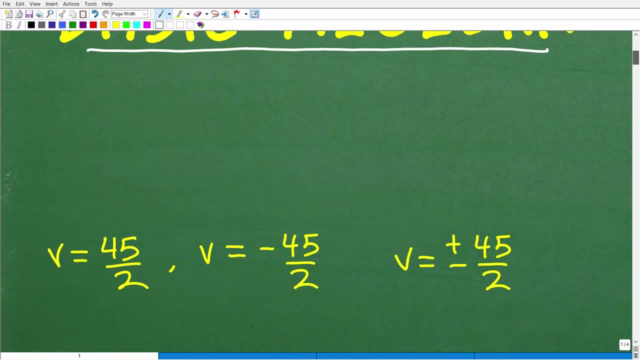 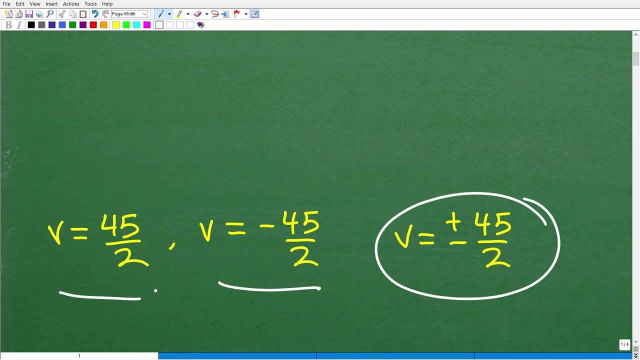 Okay, so hopefully you knew that. Let's go ahead and take a look at the answer to this equation. and there you go. So v is equal to positive negative 45 over 2.. Of course, you can write that solution this way as well, All right, so how did you do? Well, if you got this, 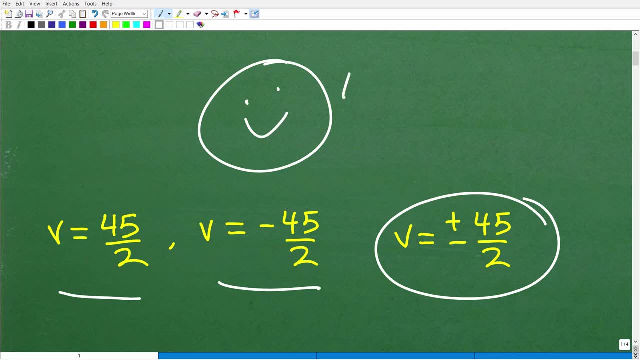 right. that's very impressive. Certainly, you definitely earned yourself a nice little happy face, an A plus a 100 percent and multiple stars, So you can tell your friends and family that you know how to solve an absolute value equation. Nice job, Okay. so let's go ahead. 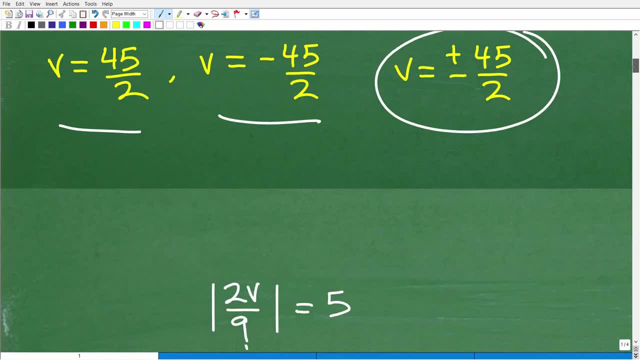 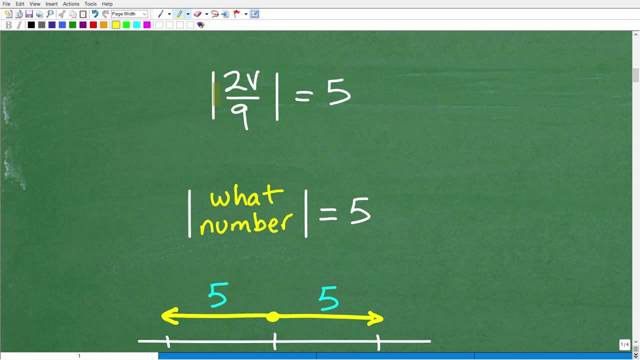 and get into this, and if you're struggling with absolute value equations, I'm going to do my best to make this very easy for you. All right, so here is our absolute value equation. I'm going to go ahead and show you how to solve it, Okay, so here's our absolute value equation Again. 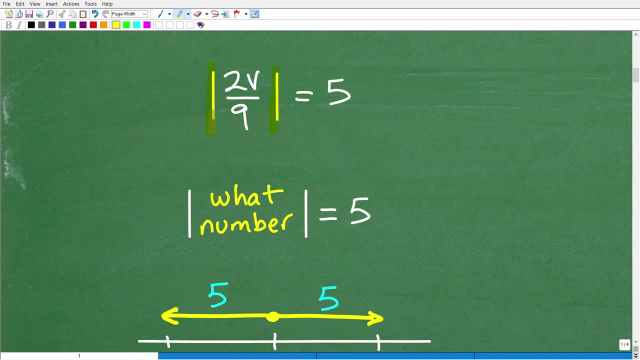 we have these little bars right here. That means absolute value. We're trying to solve for this variable v inside these absolute value bars, right, And of course this is an equation. So before we get into this actual equation, let's just kind of have a simpler form of this equation. 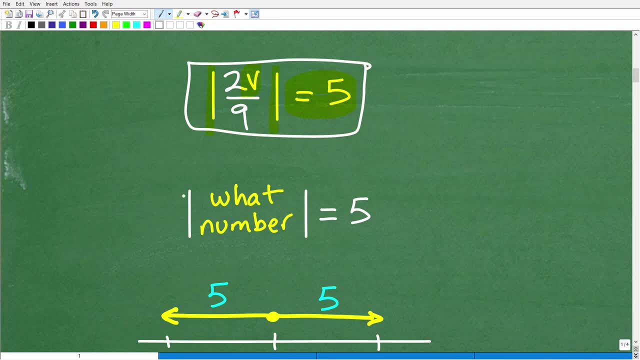 Okay, what if I told you this: Hey, what number. I have some number here, and when I take the absolute value of it, I get five. right, Some sort of mystery number, I don't know what it is, but when I plug it into my absolute value function here, I get five. So let me ask you, okay, 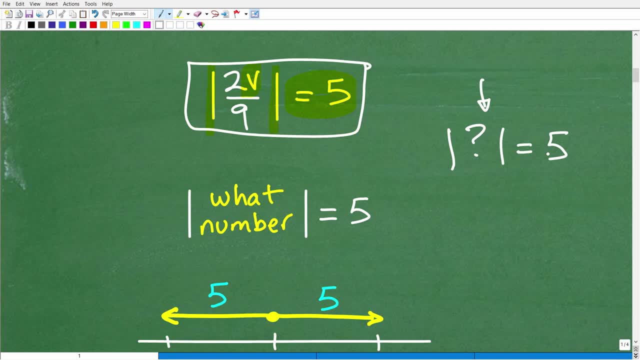 if you had to answer that little riddle or puzzle or that little question, could you do it? Okay, think of some number. When you take the absolute value of it, you get five. Now some of you might be saying to yourself: what about like negative five If I take the absolute? 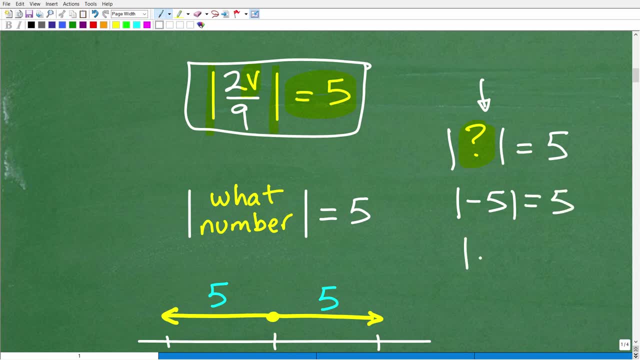 value of negative five. don't you get five? Yes, that is true. How about the absolute value of five? Do you also get five? Yes, that is true as well. So hopefully you understand that when we take the absolute value of negative five, you get five And absolute value of five. 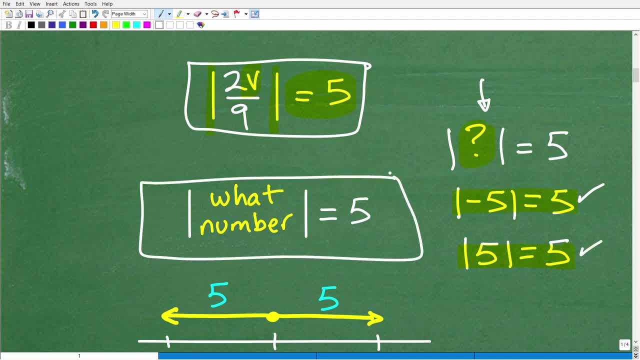 you also get five. So, going back to my little question here: the absolute value of what number is five? Well, it looks like when we take the absolute value of negative five and five, we get five. So that would be what this number could be: five or negative five. But let's. 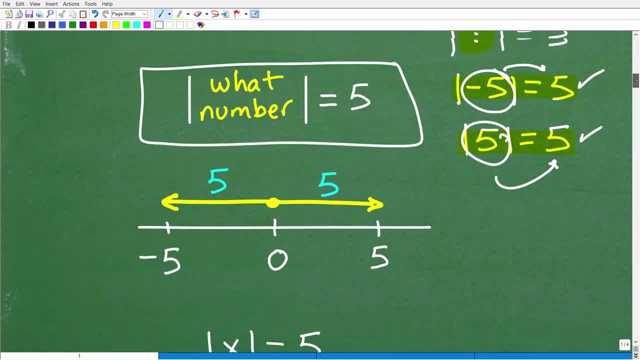 kind of look at the absolute value's definition. So what is the definition of absolute value? Well, the definition of absolute value is the distance a number is from zero on a number line. okay, So here's my little number line here: Here's zero, here's five and here's negative five. 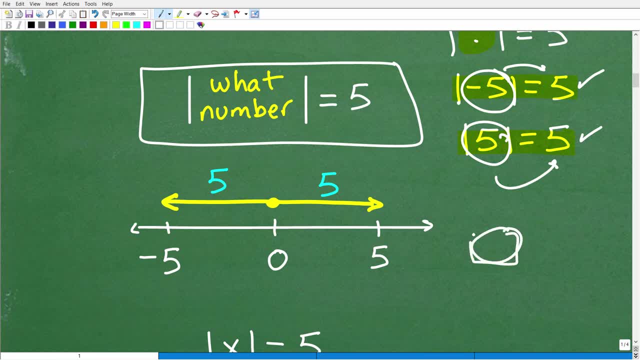 So distance, think of it like getting your tape measure out. So here we have your little tape measure, your ruler right, And we want to measure the distance. So I want to go from zero to five and I'm saying, okay, hey, how far is five from zero? You would. 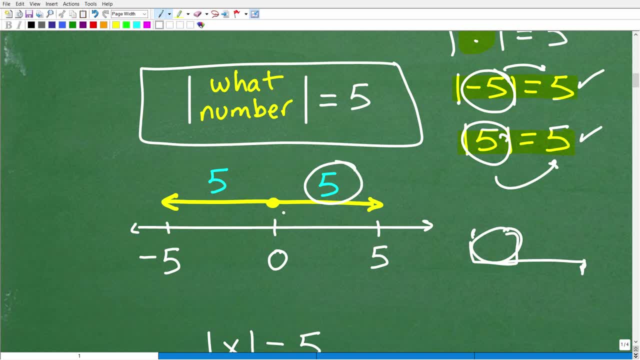 say five units away. So I say, okay, great, Measure from zero to negative five and you would tell me five units. See, when you measure like a room or some sort of like a window or a door or something like that, when you measure, okay, if you think about your little tape measure or your ruler or 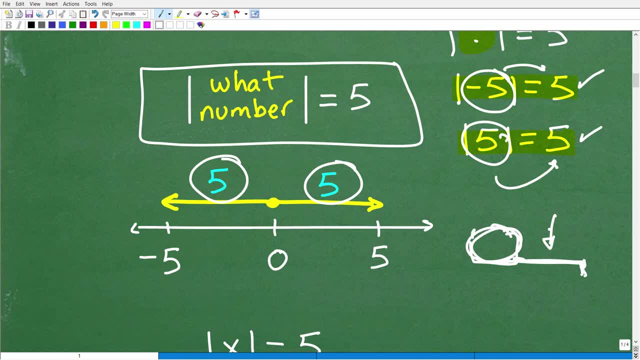 whatnot. you know you're going to be measuring in positive units. okay, Distance is typically or displacement in positive units. So five and negative five happen to be the same distance away from zero. They're just going in different directions but in terms of their distance, 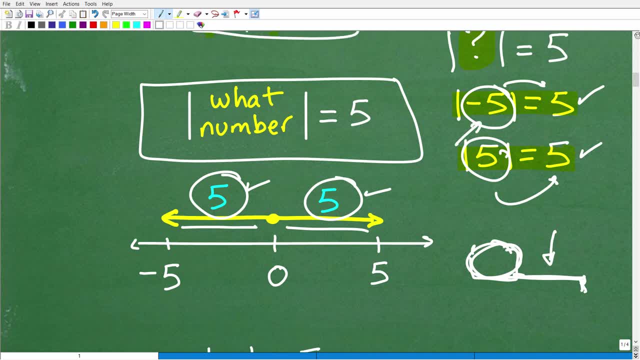 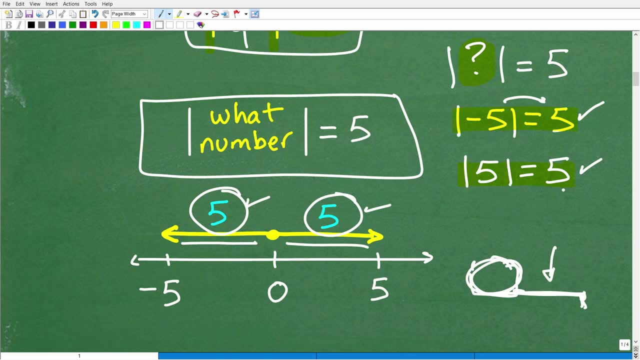 they are the same. That's why, when you think about absolute value like here- you know the absolute value of negative five is five and absolute value of five is five- You can almost think of this question as this: hey, how far is negative five from zero? 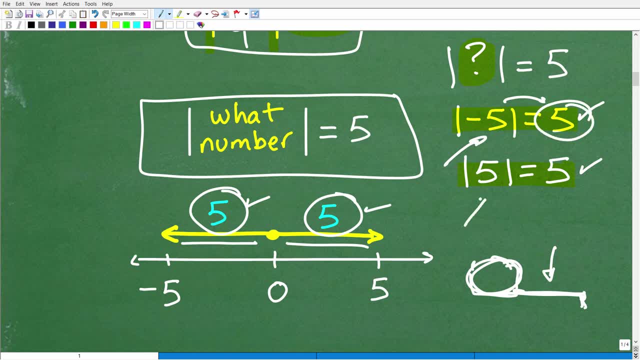 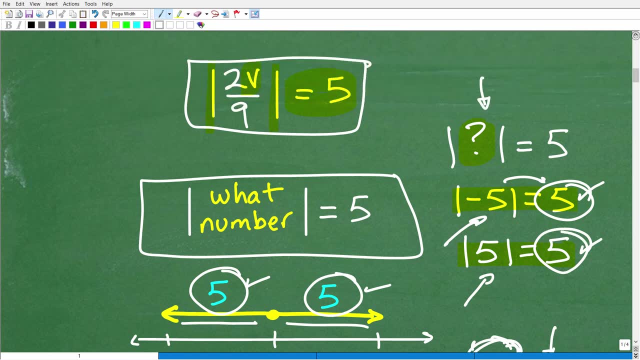 How far is negative? five from zero? Oh, it's five units away. How far is five from zero? It's also five units away, Okay. so it's really important that you understand the concepts involving absolute value, because you know, I could just tell you how to solve absolute value equations, but if you're 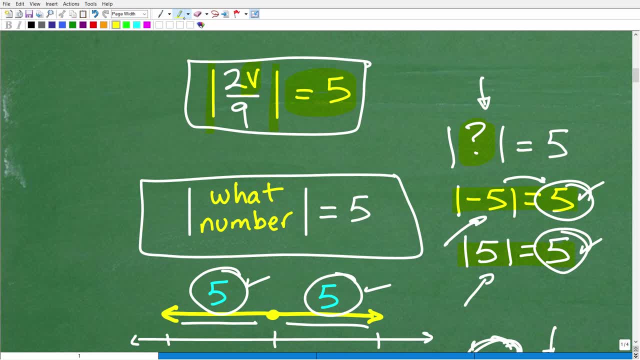 not understanding the underlying concepts, then you're going to get confused with other things. All right, so now let's go back to our equation here, and I'm saying: absolute value of 2v over 9 is five. Okay, so if you think about it, you're like 2v over 9.. What is this thing equal to? Well, 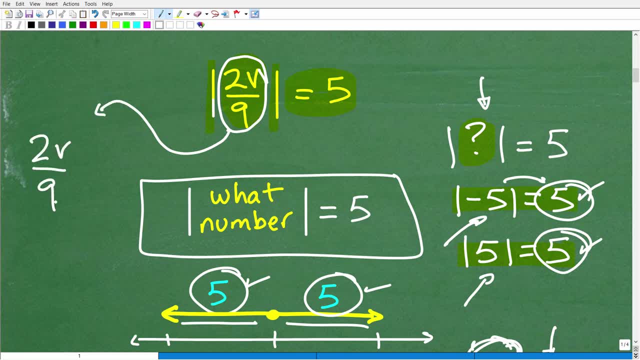 I'm like: oh, I know, 2v over 9.. I know you're just trying to disguise yourself because you must be a five or a negative five. Okay, it's the same thing. This right here must represent a five or negative five, because that's the only thing that we can plug in into this absolute value. 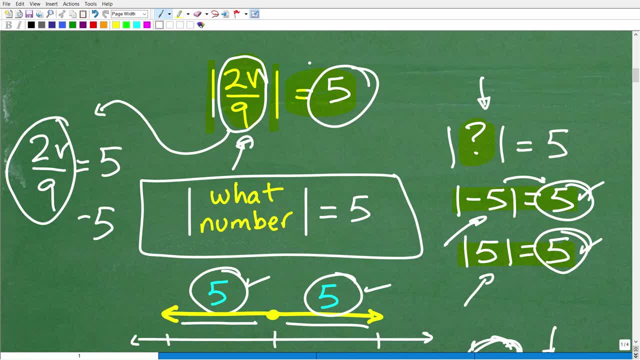 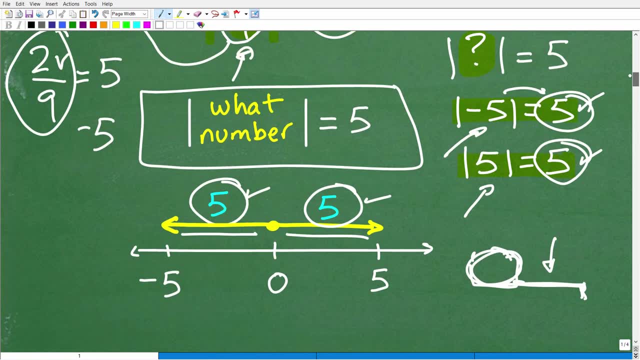 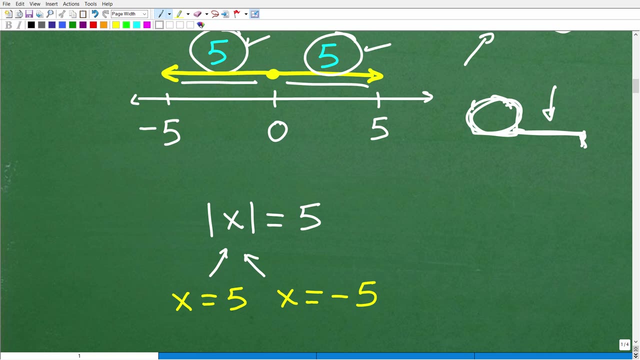 function that will make this answer come out as five. Okay, so what we want to do here is set up- let's just kind of go back here to this equation: the absolute value of what number is equal to x? Well, you could write that as this equation: absolute value of x is equal to five. 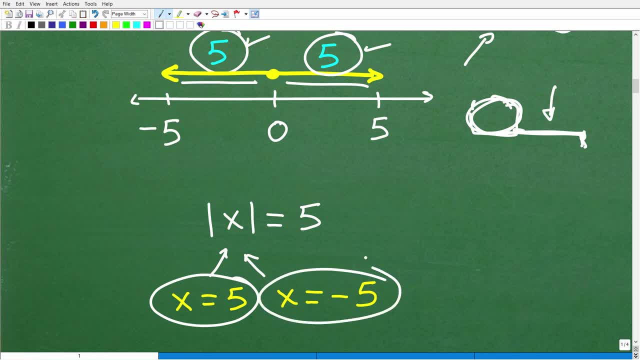 Okay, so x can either be equal to five or negative five. Here's the main thing I want you to know: When you're dealing with absolute value equations, there's always going to be two solutions. Okay, always two solutions, because you can measure out in both directions. Okay, All right. 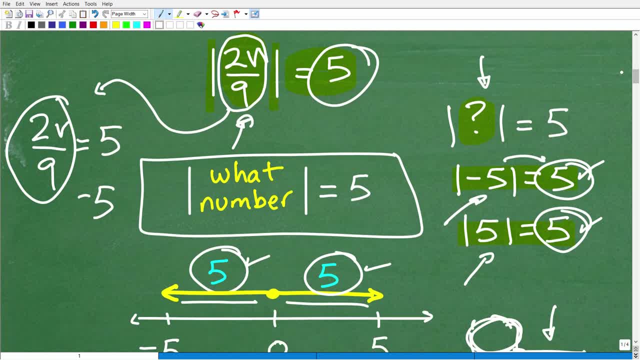 so, going back over here to this equation, okay, what you want to do is just kind of use your- you know- common sense and be like: okay, whatever's inside the absolute value equation must be equal to this number or the negative of it. Okay, and that is the exact steps you need. 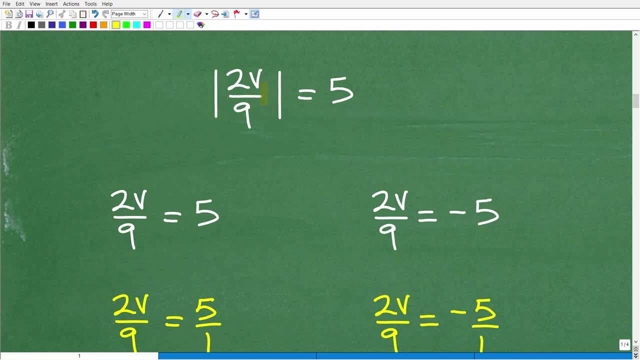 to take when you're solving an absolute value equation. All right, so you're like: okay, this is absolute value, This is equation. You're like, oh, 2v over 9, you must be equal to five or negative five. That's the only way we can get this as an answer. So set up. 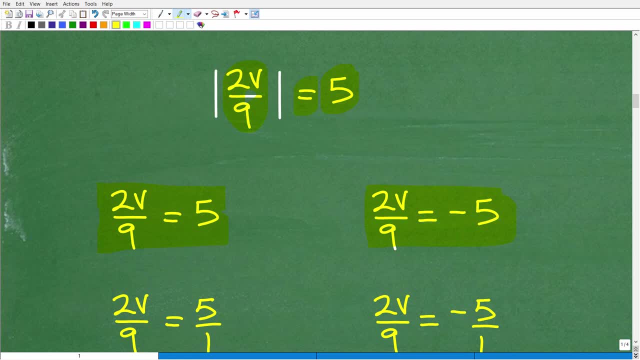 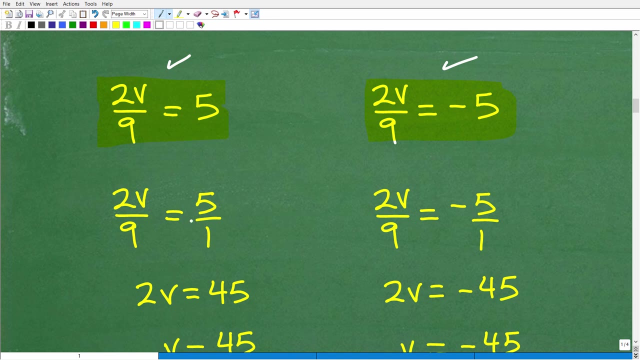 two equations. This is how you're going to get your two solutions: 2v over 9 is equal to five, Okay. or 2v over 9 is equal to negative five, And then you're going to resolve those respective equations. All right, hopefully you have basic algebra skills here. So 2v over 9, we can write. 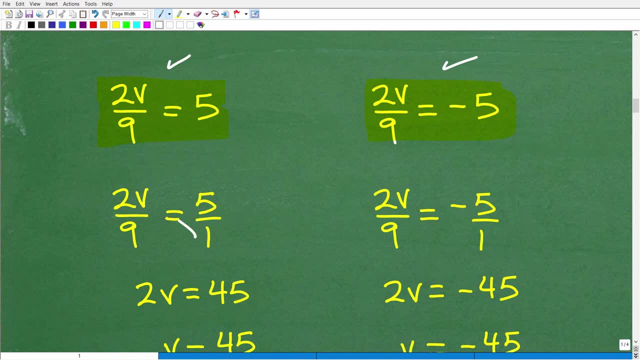 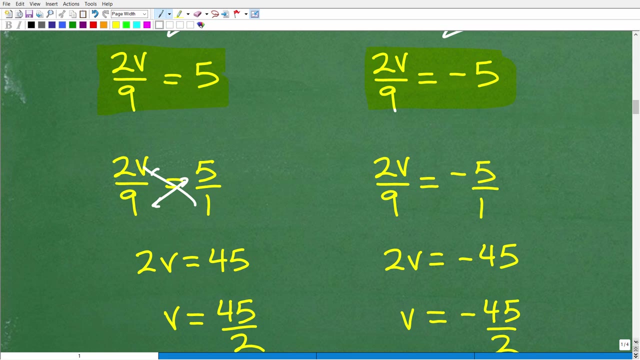 that as being equal to five or five over one, And just simply use the cross product to solve this. There's other ways you can approach this. Hopefully you have those basic algebra skills down. We are talking about basic algebra. So we have: 2v is equal to 45v is equal to 45 over. 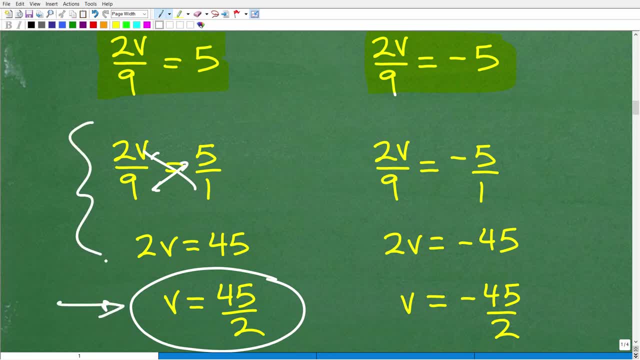 two. Now, if this part of the problem is a little bit confusing to you, then you need some assistance. You need to kind of brush up on how to solve basic linear equations. Okay, and I'm using the word basic because we're talking about pre-algebra level stuff, But listen, I'm saying the word. 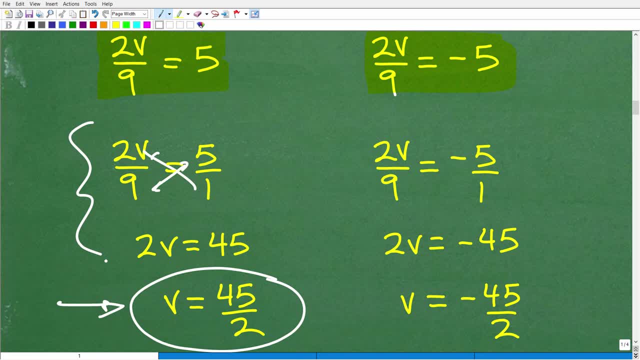 basic. but if you don't understand, you know what's going on. well, it's not basic to you, right? You're like: well, it's basic to you because you know a lot of math. it's not basic to me. Listen, I totally get that. Just trying to say that. 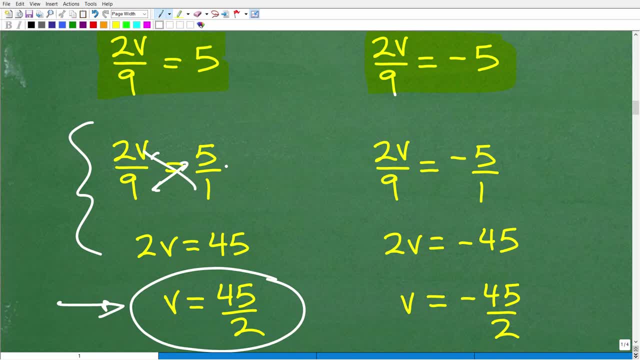 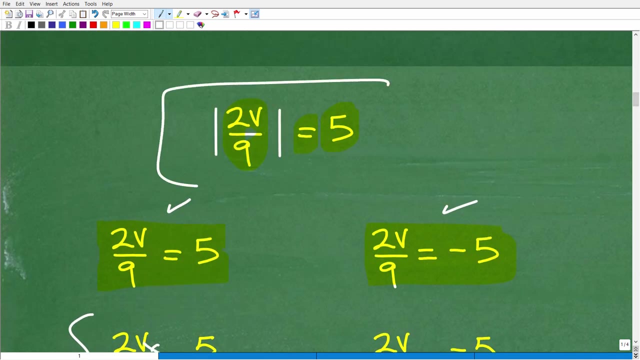 if you can't do this, this would be considered kind of like basic algebra skills, So linear equations. you got to brush up on this. And when we solve for v in this equation we're going to get, v is equal to negative 45 over two. All right, so some final thoughts here. Okay, when you are 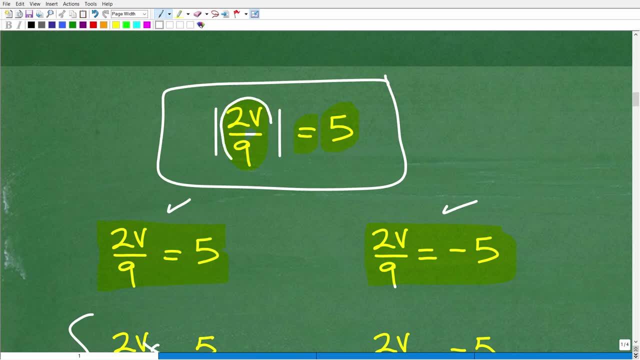 solving an absolute value equation. whatever that expression is on the inside. okay, it's going to be positive and negative of this number. Okay, you need to know these steps And you could have more involved, more interesting absolute value equations. Let me just show here. So if I had two, 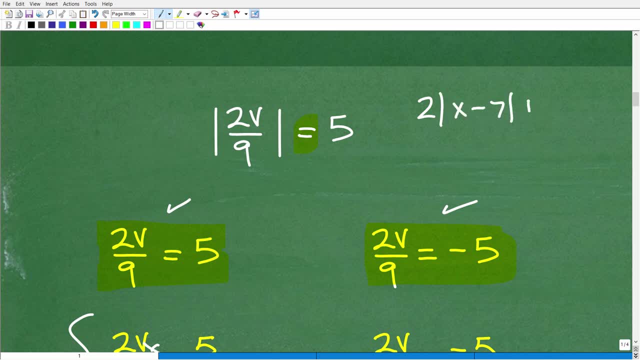 times x minus. the absolute value of x minus seven plus one is equal to, let's say, six. All right, well, we can't set up the two equations until I kind of isolate this absolute value part. Okay, so this is a very basic absolute value equation. In this case I'd have to subtract one from both. 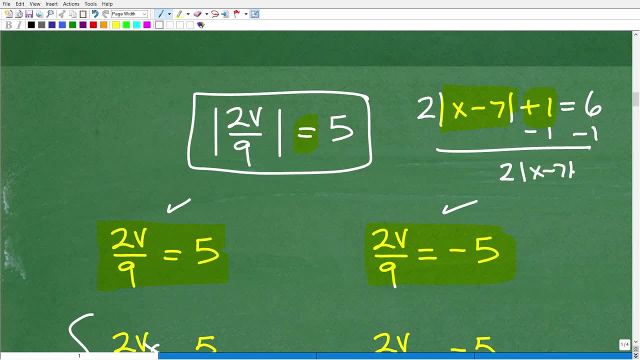 and then I'm going to end up with two times absolute value of x minus seven is equal to five. then I need to divide both sides of the absolute value equation by two, So I get x minus seven is equal to five halves. Now I need to set up okay to have my two separate equations here.